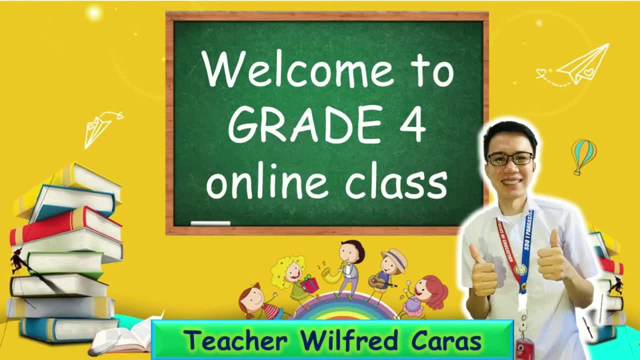 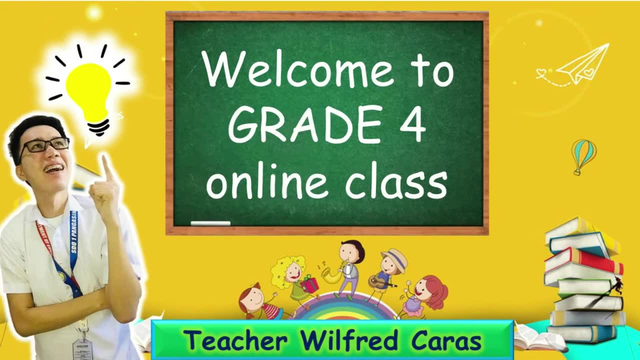 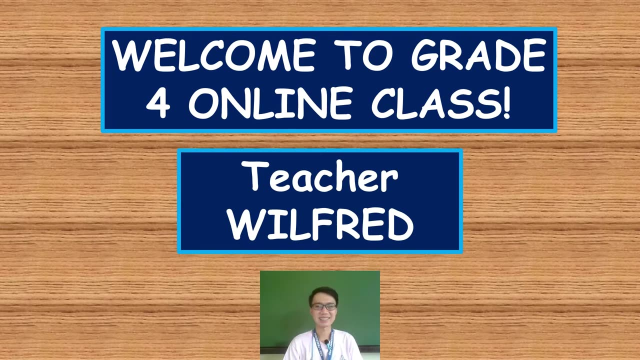 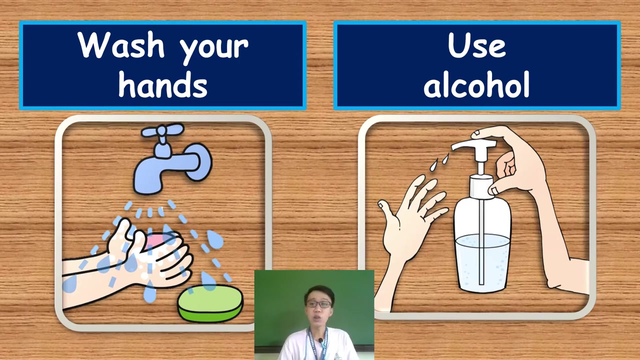 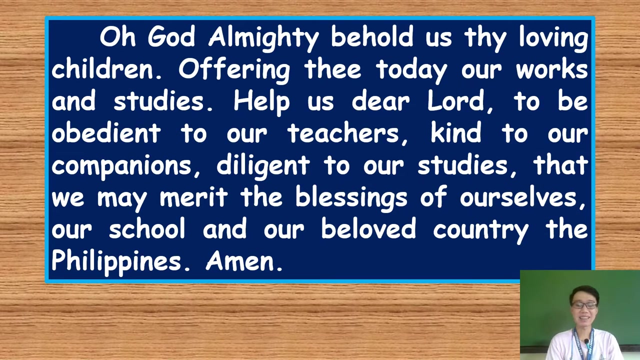 Hi, Before we start the class, kids, let us bow our heads and feel the presence of the Lord. All God Almighty, behold us thy loving children offering day to day our works and studies. Help us, dear Lord, to be obedient to our teachers, kind to our companions, diligent. 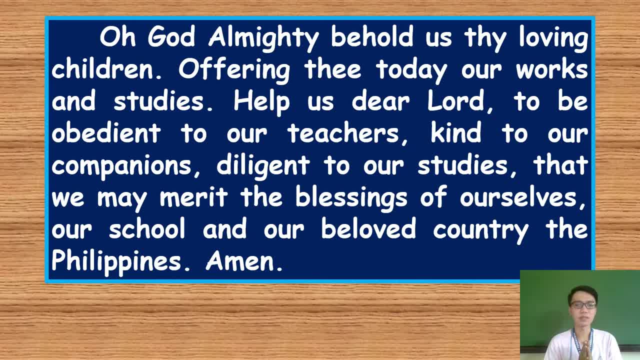 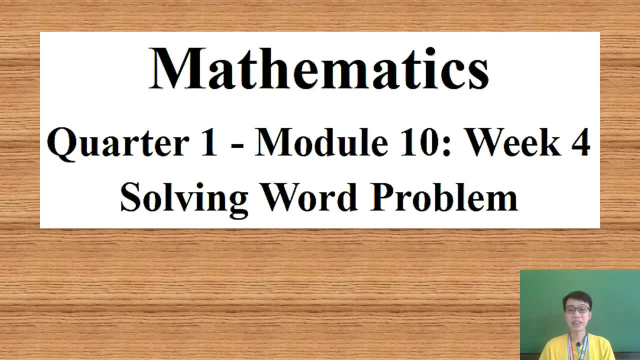 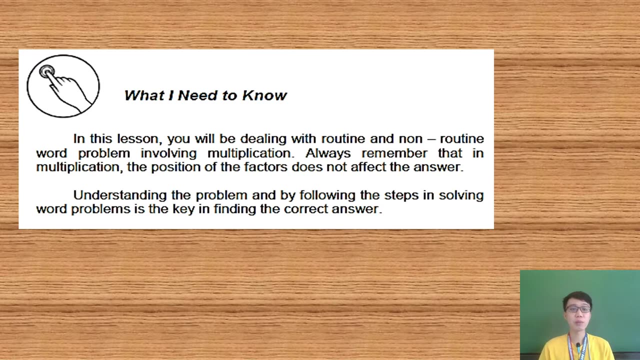 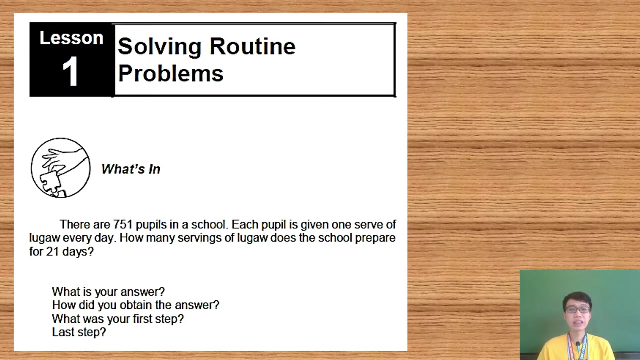 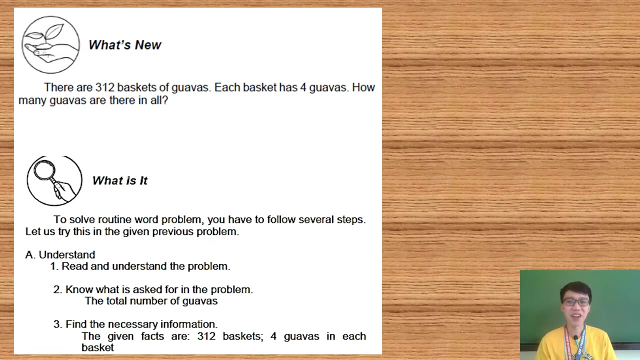